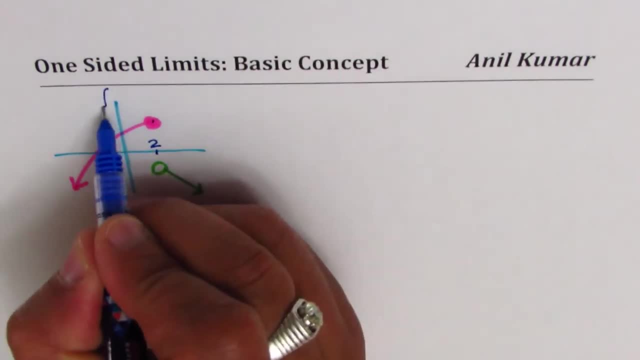 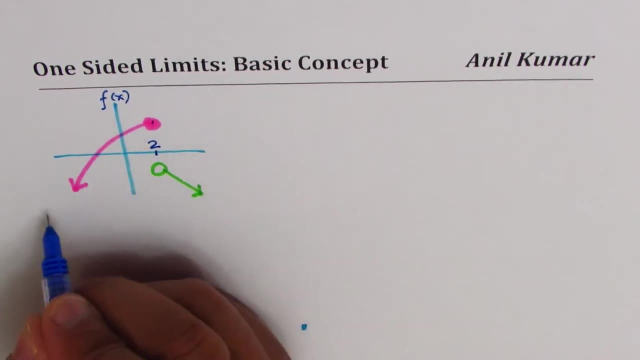 jump discontinuity. we'll call this function as f of X. now the question here is: what is the limit of this function when X approaches 2? from the left side, and we'll call this as the left side. okay, from the left side, which we write with negative exponent. so what is the limit of this function when? 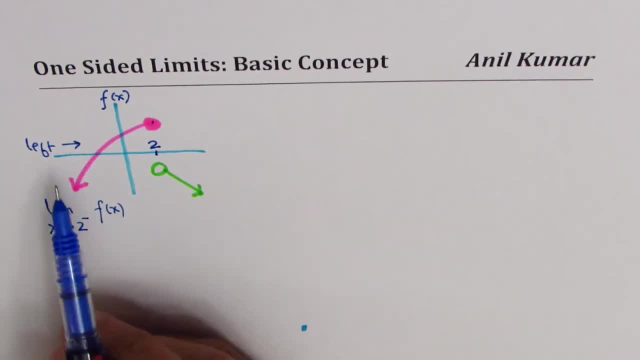 X approaches 2 from the left side. now, since we are approaching only from one side, we call it one-sided limits. is it okay? okay, the answer for this is: when you approach from this side, you actually hit this part of the graph, and where you reach is its limit. let's say this value which 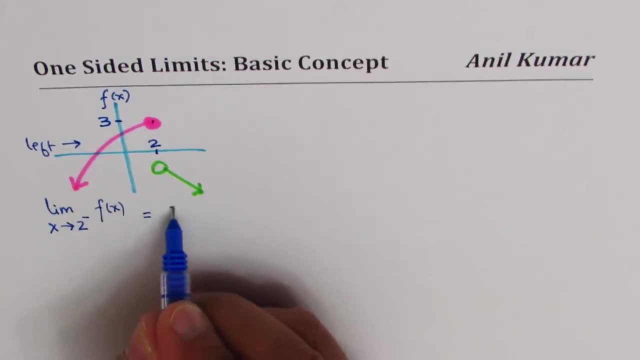 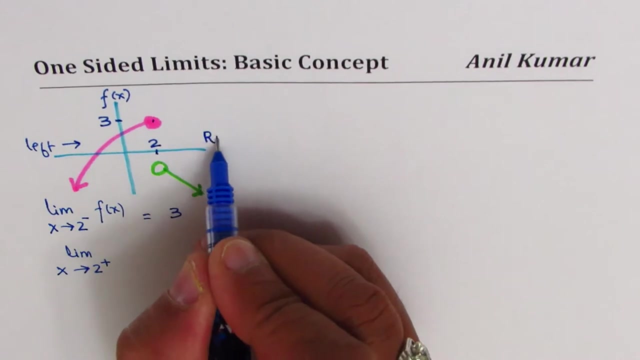 you are approaching is 3, then the answer will be 3. is that okay? I could have asked a different question. what is the limit of this function when X approaches 2 from the right side? and that right side is indicated by plus sign. so this is your right side. 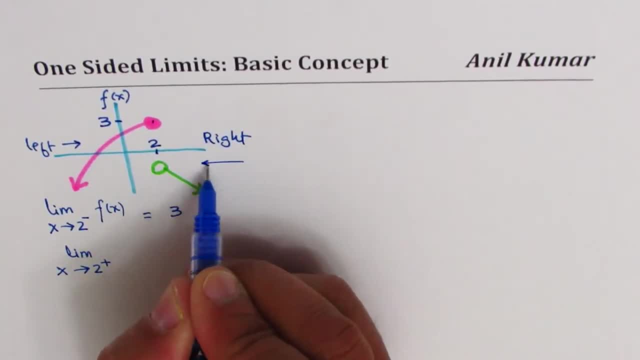 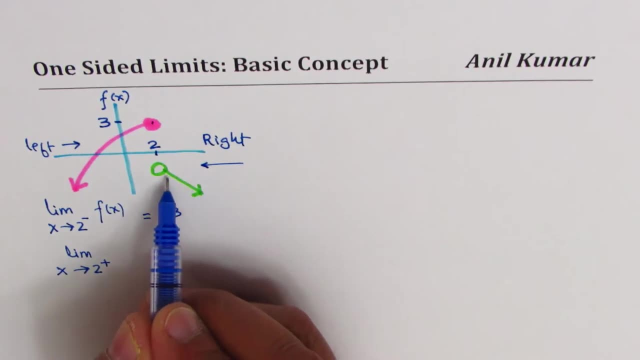 so if I approach from the right side, I'm going to hit this part of linear curve and I'll approach this value as I come closer and closer to 2 right. let's say this value is minus 2, so the value of this function or the limit of this, 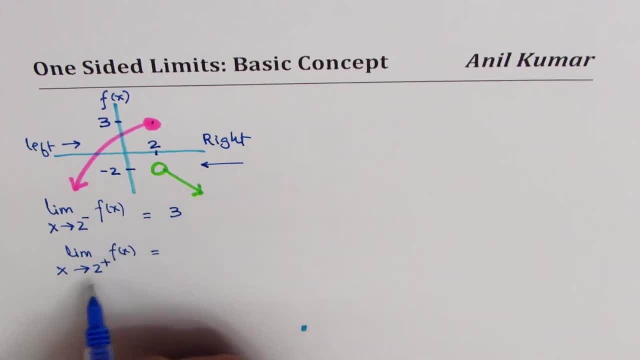 function. as X approaches, 2 from the right side will be minus 2. so that is what we consider one-sided limits: limit from either side. now you have been doing limit when X approaches a value, let's say 2. now, in this particular case, if you approach true from left side, you 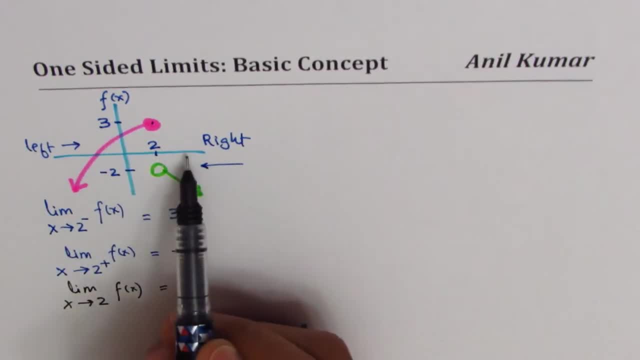 reach at 3. if you are approaching 2 from the right side, you are approaching minus 2. they are not equal. so when they are not equal we say the limit does not exist. the reason is these two limits are not equal. I hope you got the concept right now from the 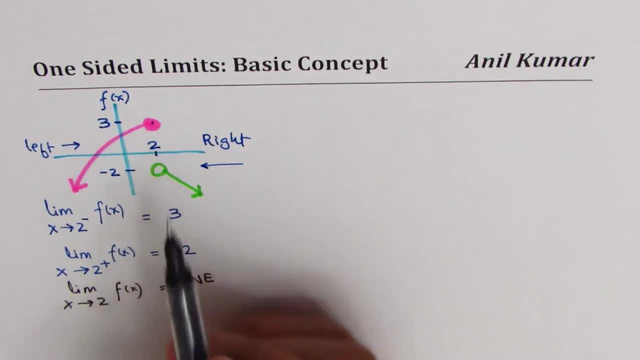 graph. at times you may be asked to find the value of the function at 2, which, let me write as: what is f of 2, equal to that filled in hole here, gives you the value which is 3, is it okay? so that is how you're going to answer one-sided limits based questions, if a graph is given to you right now? 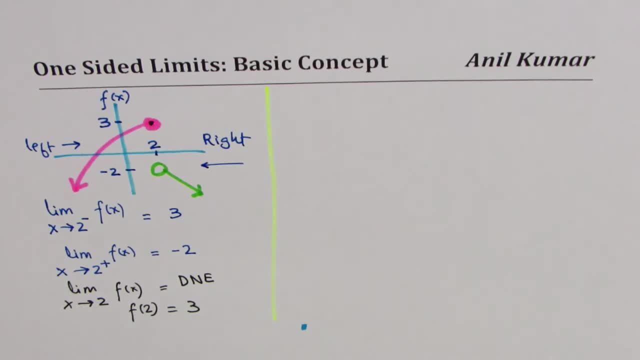 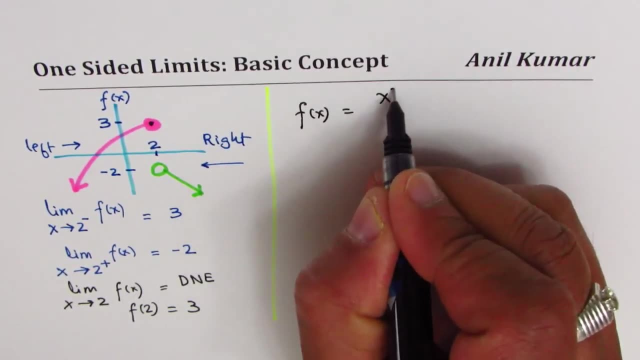 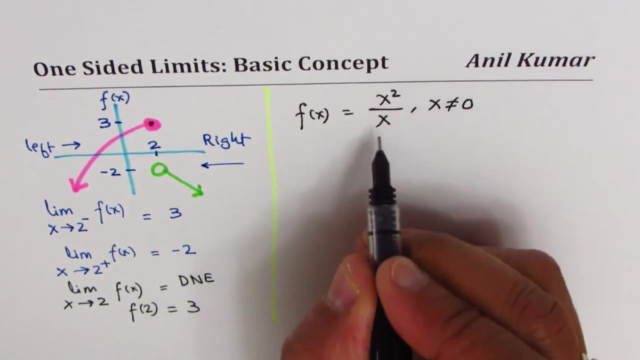 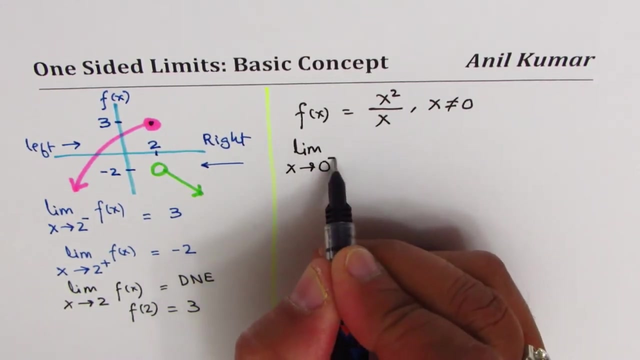 let me take another example. so let's take an equation this time. so so we have a function f of X which is x squared divided by X, as you can see from here that X should not be equal to 0, because then it is not defined, is that okay? so for this particular function, you need to find limit as X approaches 0 from the left. 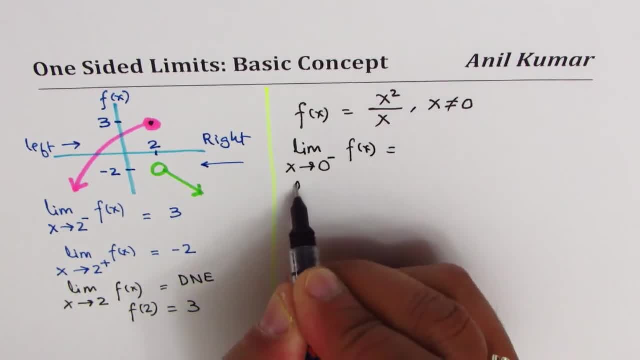 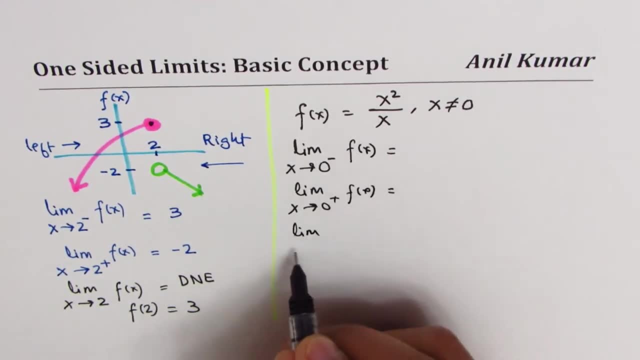 side that is minus. you need to find the limit when X approaches 0. from the right side for the same function. you need to find the limit when X approaches 0. right, let's check it out. well, the best way is to really sketch it and then write down the answers. so let's sketch it here and we'll write down the. 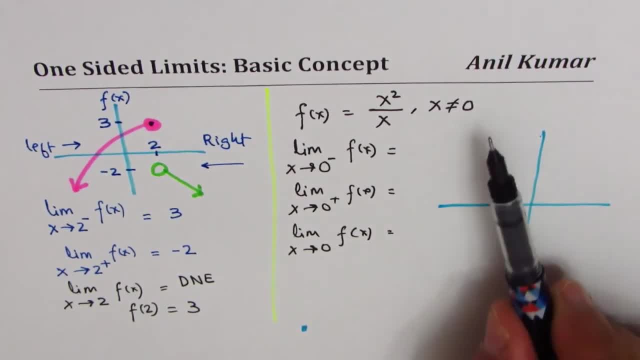 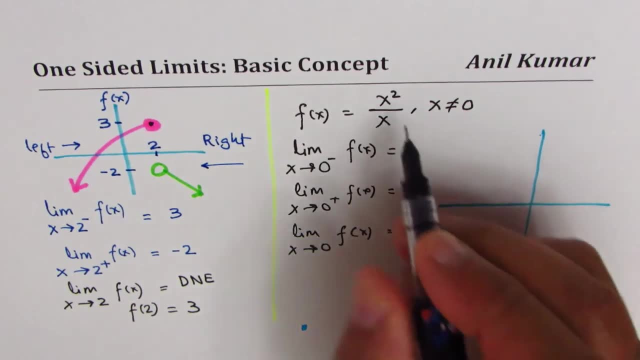 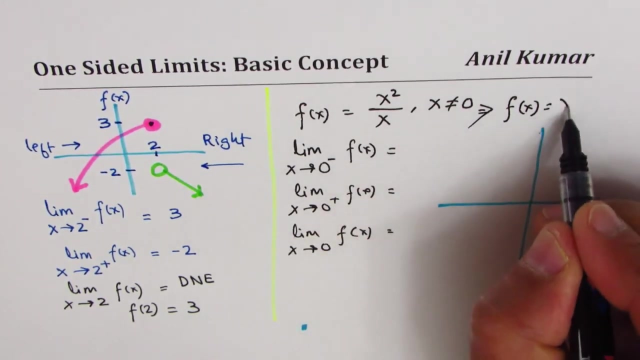 answers. so of course, at 0 it is not defined. so this function could be written as if I cancel one of those X's. so we write this as f of X is equals to X where X is not equal to 0. does make sense to you? yes, it does. 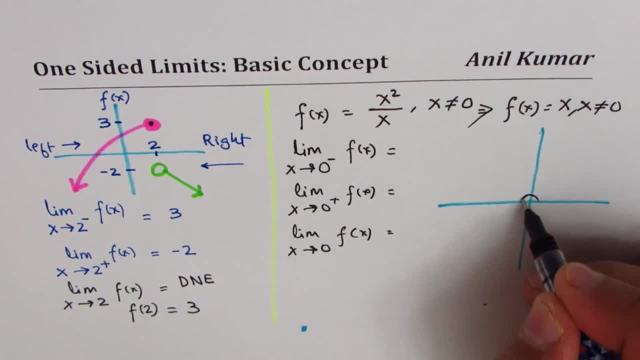 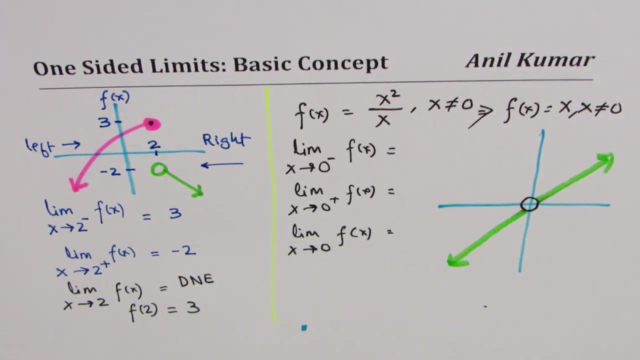 right. so basically at 0 we have a whole and the function could be grapht as X, perfect, so that becomes the given function, and now it's easy for us to answer all these questions. so sketching is a good way of doing things for finding one-sided limits. okay, so when you're 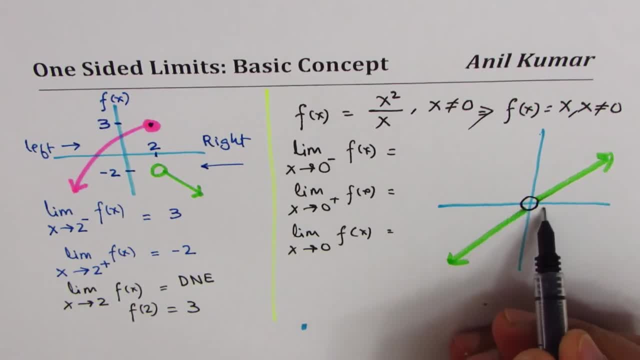 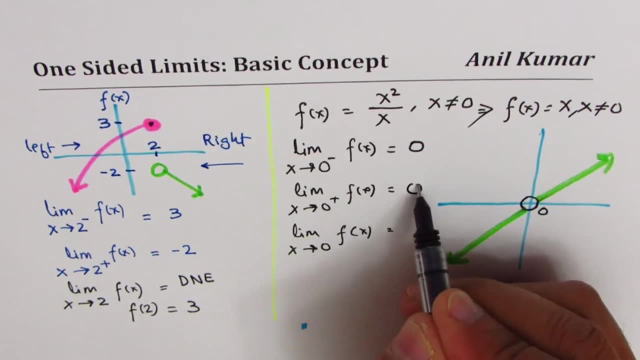 approaching 0 from the left side, you hit this portion and you're approaching a contribution measure called f, as in the哥 0 itself. So this answer is 0.. If you are approaching from the right side, you again approach origin, so it's 0.. Since these two limits, from left and right, are same, the limit